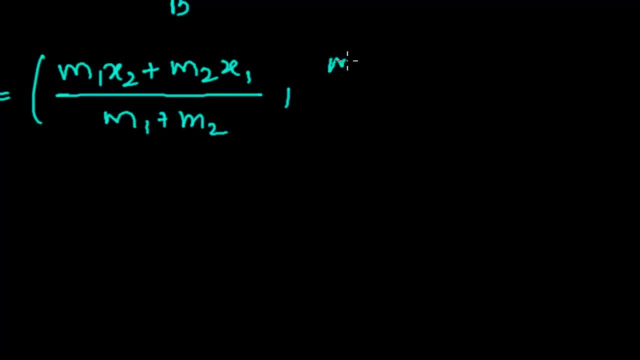 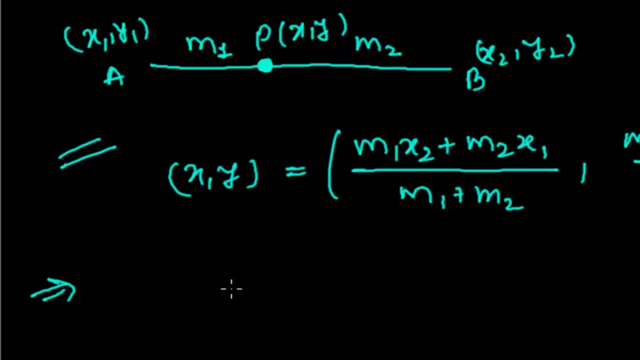 This is X coordinate and the Y coordinate is again M1Y2, right Plus M2Y1, whole divided by M1 plus M2, right. This is the section formula We recently learned. This is in some ratios right. Now let's observe a particular condition, right, Suppose this is a line, again the same line. This is A line which has X1, Y2, B. 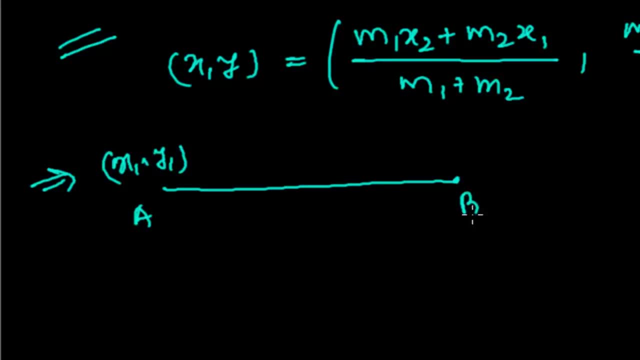 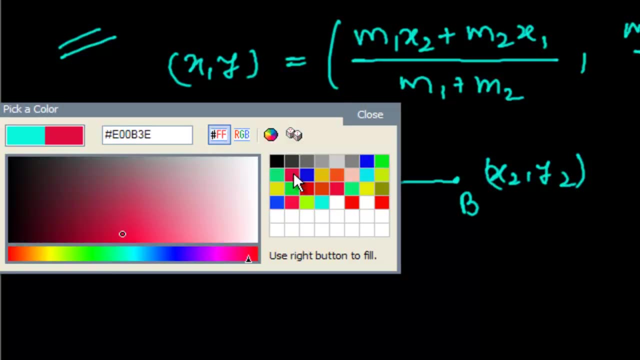 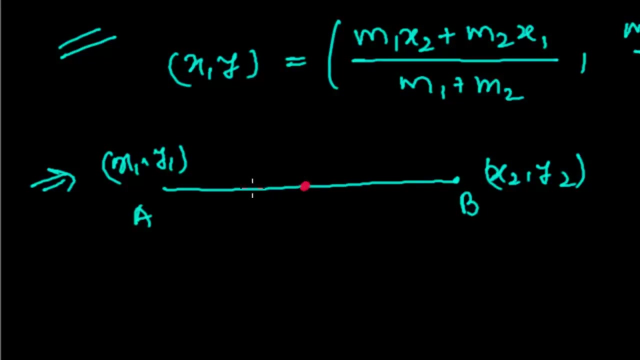 And this is B line which has X2 and Y2, right, Coordinate. Now, let's suppose, let me do with this color. fine, This is now point P, exactly at the midpoint, right, Exactly at the center, Exactly. Means: this is P point now And its coordinate is now, let's say it's XY again, right, But it is exactly equal, right. Means: AP is equals to this AP. 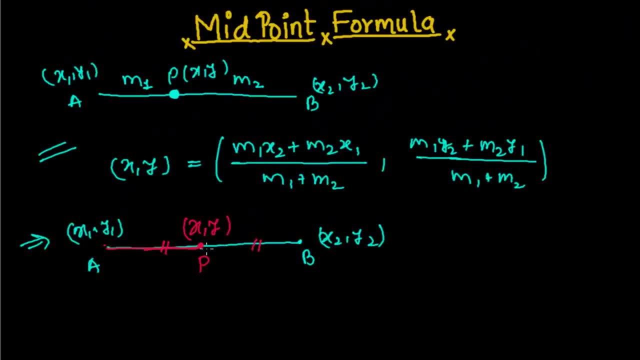 AP distance is exactly right, Exactly equals to PVD distance. So it is exactly at the middle point, right. So now, what is the coordinate or what is the formula to find out? this coordinates, right Now, what we can say, in this condition that this P point is dividing this AB in one ratio, one right. We can simply say it because, see here this part and this: 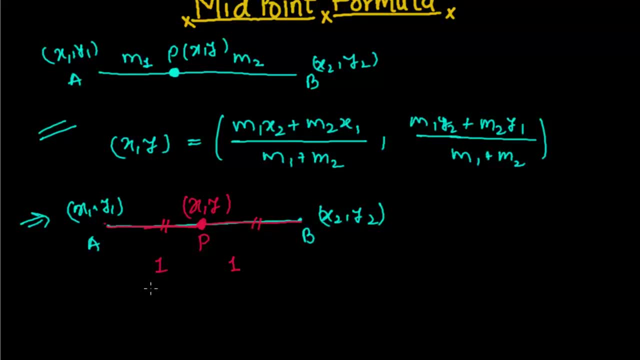 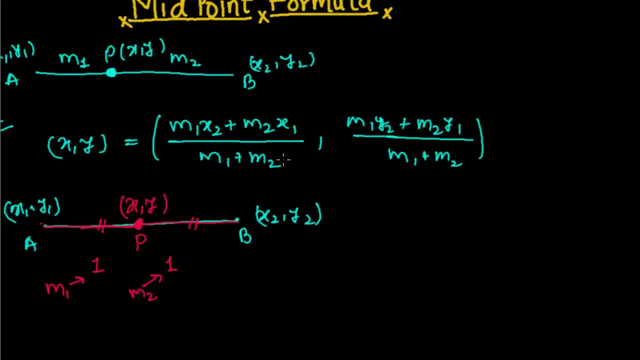 part are equal. So let me suppose here, I don't have to suppose even, because here M1 is one, again and again M2 is also one, right. So it's a ratio of M1 used to M2, right. So now let me find the value of XY by using this M1 and M2 here, right. So again, here XY will be right. See this, M1, right, M1 is one. This is X2. again, M2 is again one, And it is. 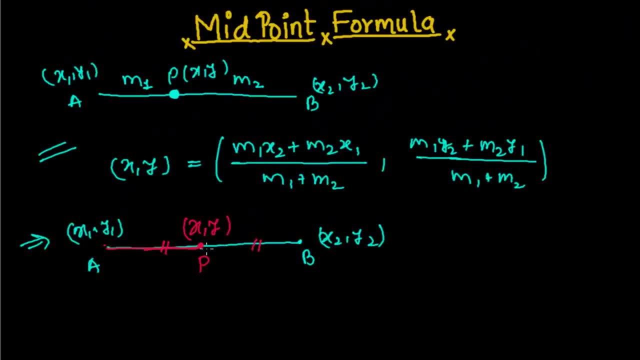 AP distance is exactly right, Exactly equals to PVD distance. So it is exactly at the middle point, right. So now, what is the coordinate or what is the formula to find out? this coordinates, right Now, what we can say, in this condition that this P point is dividing this AB in one ratio, one right. We can simply say it because, see here this part and this: 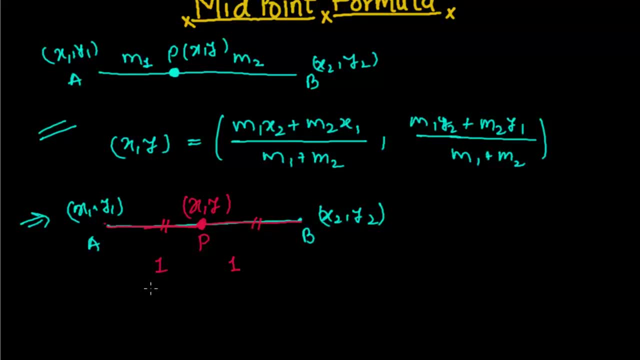 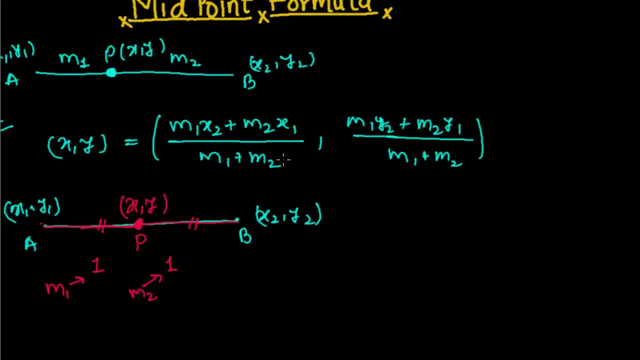 part are equal. So let me suppose here, I don't have to suppose even, because here M1 is one, again and again M2 is also one, right. So it's a ratio of M1 used to M2, right. So now let me find the value of XY by using this M1 and M2 here, right. So again, here XY will be right. See this, M1, right, M1 is one. This is X2. again, M2 is again one, And it is. 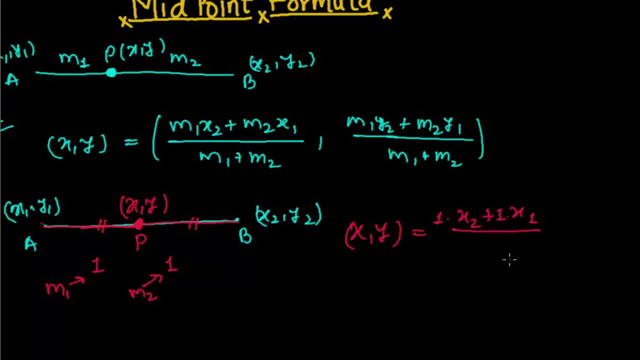 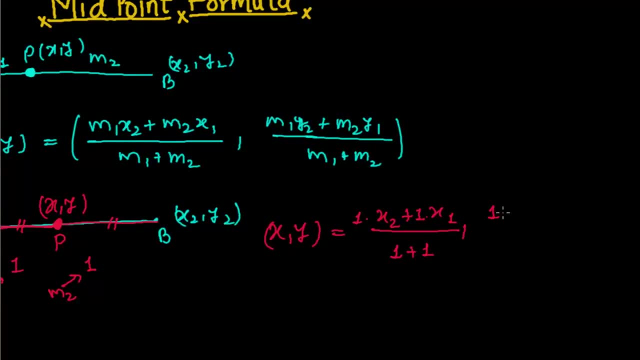 X1, right, Whole, divided by M1 plus M2, that is one plus one. And again see M1, M1 is again one, And this is Y2, right. Again, plus M2 is again one. And this is Y1, right, So Y1, it's like this. So now let's divide. So I will get: M1 is again one and M2 is again one, right, So let me close the bracket. And now what we got. 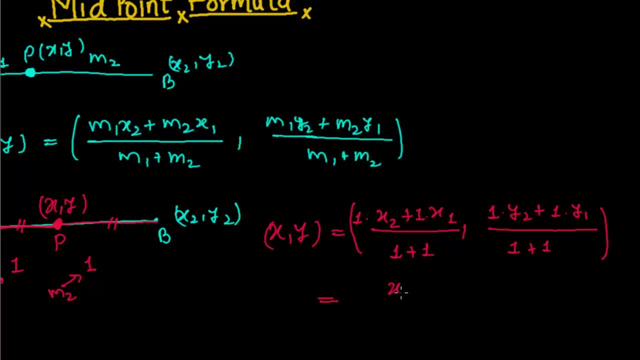 one into X2 and one into X1.. So simply, I can write X1 plus X2, whole divided by two, And again Y1 plus Y2, whole divided by two. I'm just keeping this X2 backside and Y2, this backside right. It is easy to remember one, two, one two right And one that is two two. So this point, this formula right, this XY formula, equals to this X coordinate and this M1.. 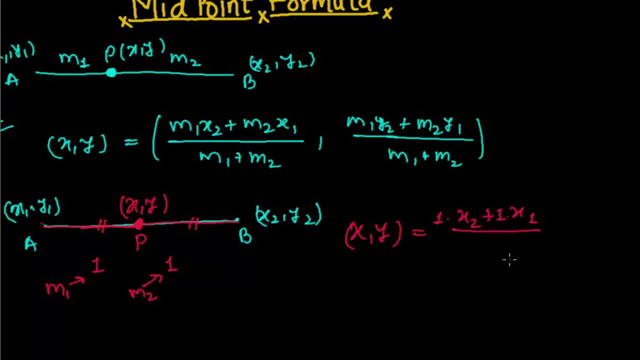 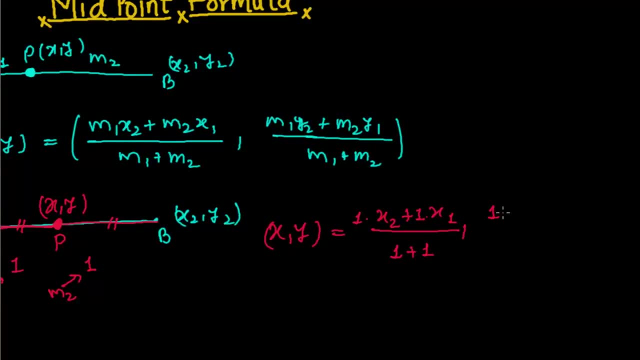 X1, right, Whole, divided by M1 plus M2, that is one plus one. And again see M1, M1 is again one, And this is Y2, right. Again, plus M2 is again one. And this is Y1, right, So Y1, it's like this. So now let's divide. So I will get: M1 is again one and M2 is again one, right, So let me close the bracket. And now what we got. 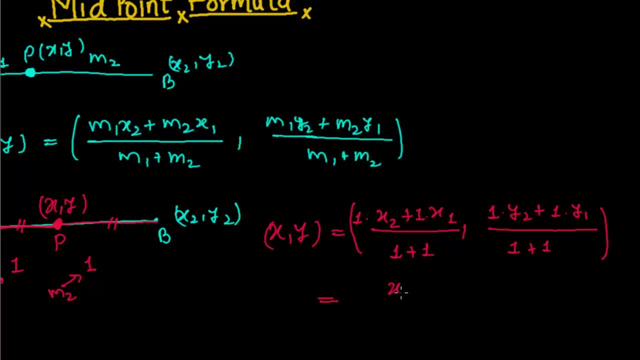 one into X2 and one into X1.. So simply, I can write X1 plus X2, whole divided by two, And again Y1 plus Y2, whole divided by two. I'm just keeping this X2 backside and Y2, this backside right. It is easy to remember one, two, one two right And one that is two two. So this point, this formula right, this XY formula, equals to this X coordinate and this M1.. 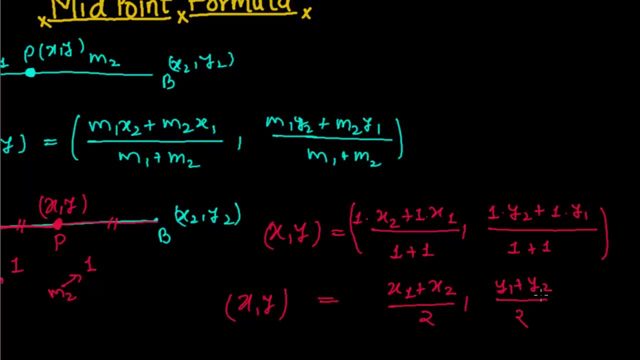 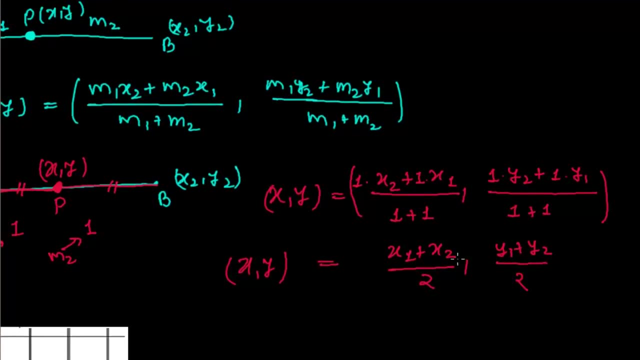 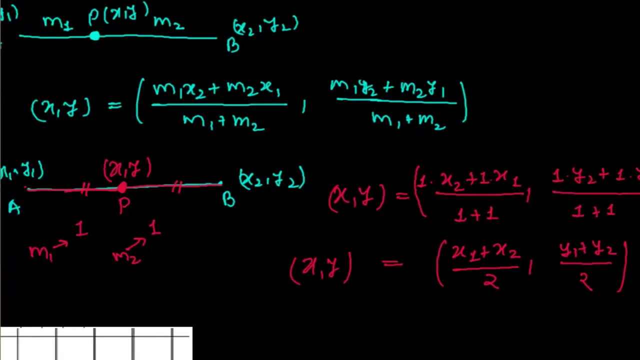 This Y coordinate is X1 plus X2 upon two or Y1 plus Y2 upon two. So what we're seeing over here there. let me tell you here this: one and two upon two, this is an average, exactly right. This is an average in. you have learned in mean median mode, that right. it's exactly the mean or average of this point, two points right Here. I mean to say this is exactly the average of these two points: X1 and X2's average is this: 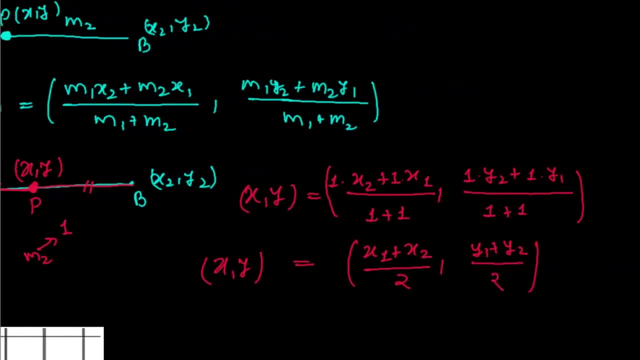 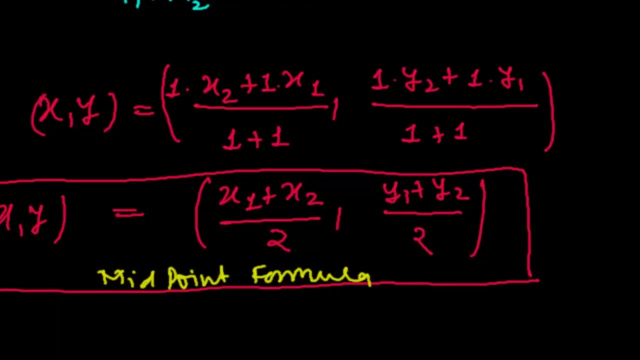 X part and Y1 and Y2's average. is this part, right? This is called the midpoint formula. exactly right, This is called midpoint formula. right, This is called midpoint formula. midpoint formula. This is exactly no more than the average average of two, right? Let me do in this figure right, I think here. 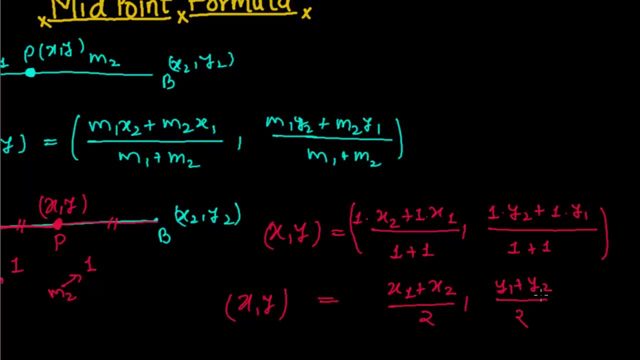 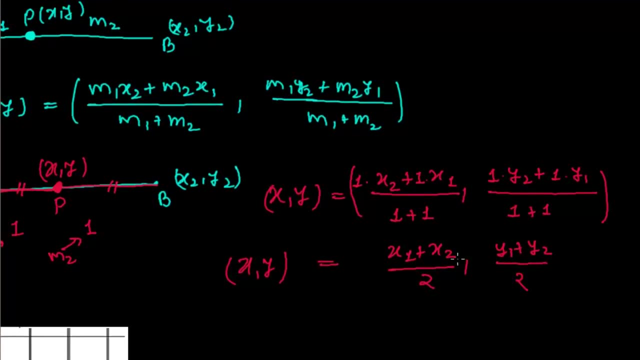 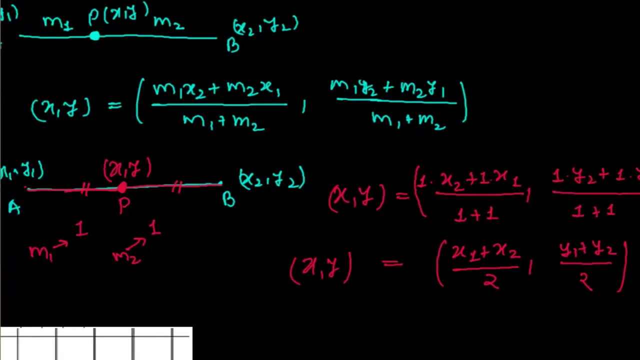 This Y coordinate is X1 plus X2 upon two or Y1 plus Y2 upon two. So what we're seeing over here there. let me tell you here this: one and two upon two, this is an average, exactly right. This is an average in. you have learned in mean median mode, that right. it's exactly the mean or average of this point, two points right Here. I mean to say this is exactly the average of these two points: X1 and X2's average is this: 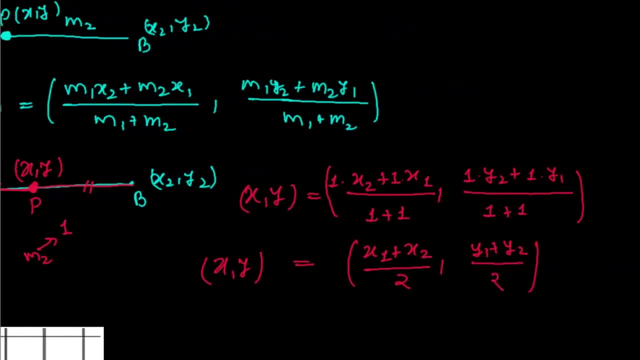 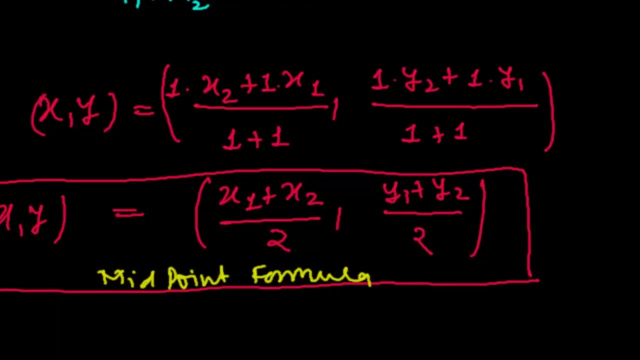 X part and Y1 and Y2's average. is this part, right? This is called the midpoint formula. exactly right, This is called midpoint formula. right, This is called midpoint formula. midpoint formula. This is exactly no more than the average average of two, right? Let me do in this figure right, I think here. 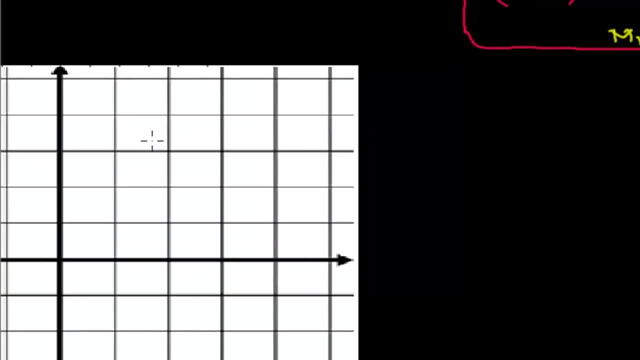 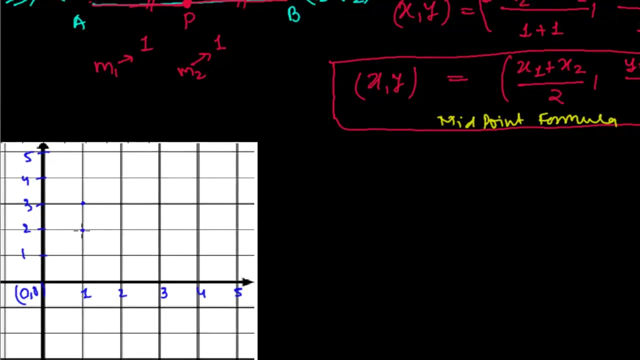 the red will be best, or this blue. okay, Suppose this coordinate, this is origin right. So it is zero, zero of course. And this is one. this is two, three, four, five. This is again one, two, three, four, five right, Suppose there is a line that suppose it is here. So it is one, two right. And here is another point, that is C. 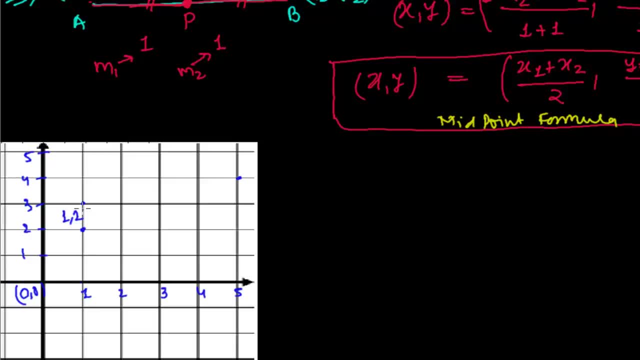 It's one and one, two, So its coordinates are one, two. And here is five, and then one, two, three, four, right. So its coordinates are five, four, right. Now I have to take the middle of this, right, exactly, middle of this. It will be about here, right? So this point is the middle of this, right, exactly. So it's exactly the average. you know, I told you already it is the average, So average of one and one, two. 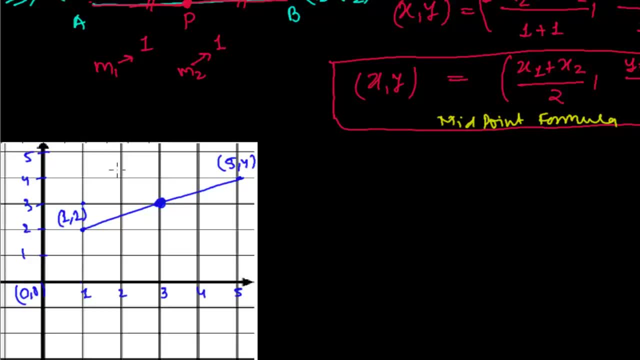 five. now i have to take what is the average of one and five. simply, i'll be: uh, average of one and five, right? so let me change the color. fine, right? so average of one and five. so i simply add this: both one plus five divided by two, that will be equals to six by two, that is three, right? 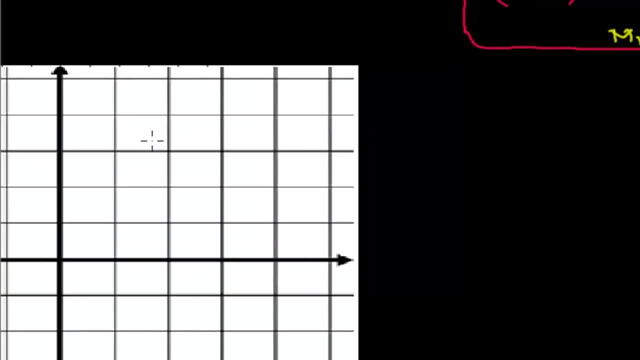 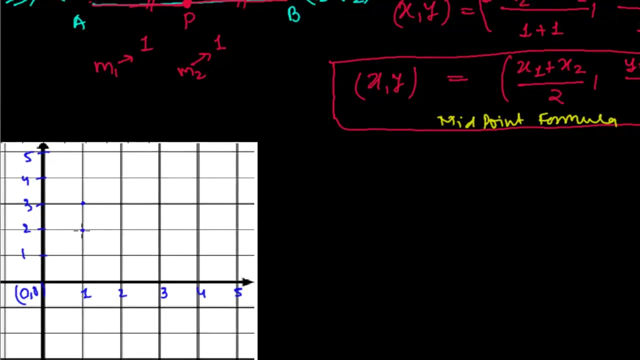 the red will be best, or this blue. okay, Suppose this coordinate, this is origin right. So it is zero, zero of course. And this is one. this is two, three, four, five. This is again one, two, three, four, five right, Suppose there is a line that suppose it is here. So it is one, two right. And here is another point, that is C. 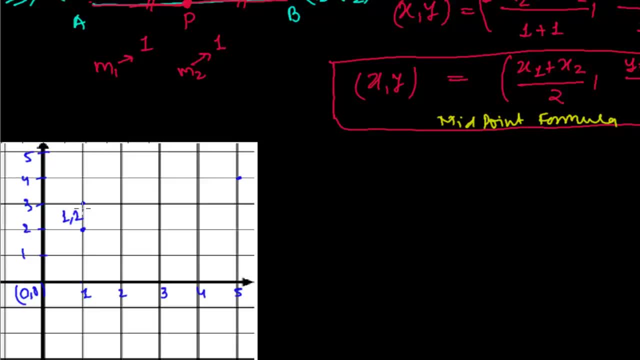 It's one and one, two, So its coordinates are one, two, And here is five, and then one, two, three, four, right. So its coordinates are five, four, right. Now I have to take the middle of this, right, exactly, middle of this. It will be about here, right. So this point is the middle of this, right, exactly. So it's exactly the average. you know, I told you already it is the average, So average, of one and one, two, three, four, five, right. So it's exactly the average. you know, I told you already it is the average, So average, of one and one, two, three, four, five, right. So it's exactly the average. you know, I told you already it is the average, So average, of one and one, two, three, four, five, right. So it's exactly the average. you know, I told you already it is the average, So average, of one and one, two. 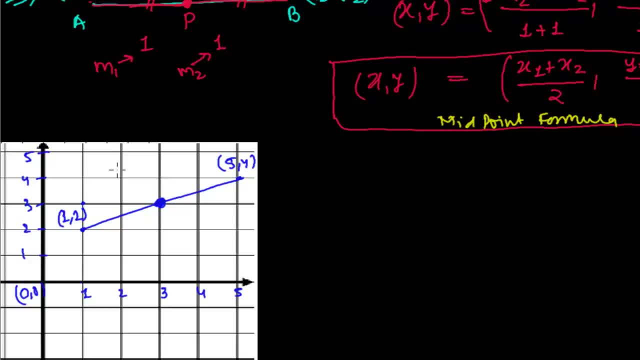 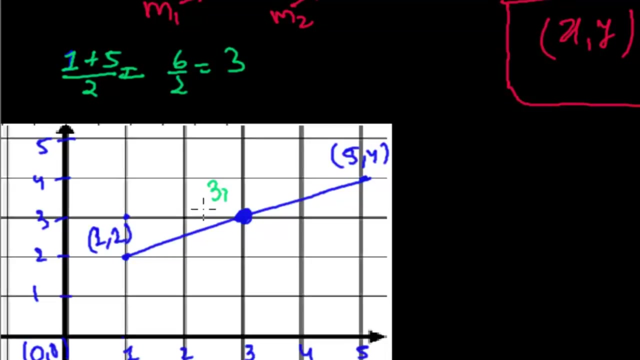 five. now I have to take what is the average of one and five. simply, I'll be average of one and five, right? So let me change the color. Fine, Right, So average of one and five. So I simply add this: both one plus five divided by two, that will be equals to six by two, that is three, right? So x coordinate is now three. Again. average of this two and four, or I can say mean of this two and. 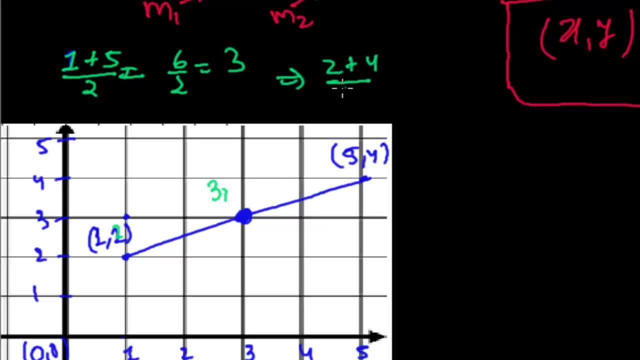 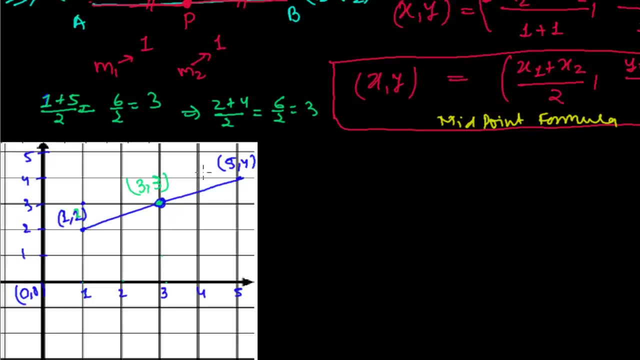 four. Again, let me take here two plus four divided by two. that is again four plus two. six upon two equals to three. So again I got the value y, value three, right. So this is also three, three. see here: one, two, three. one, two, three. So it's simply the average, right? It's a midpoint formula, it's just the average of two coordinates, right? Just take the average of the average of mean. you can say simply: if you're learning the statistics, then it's simply the mean. 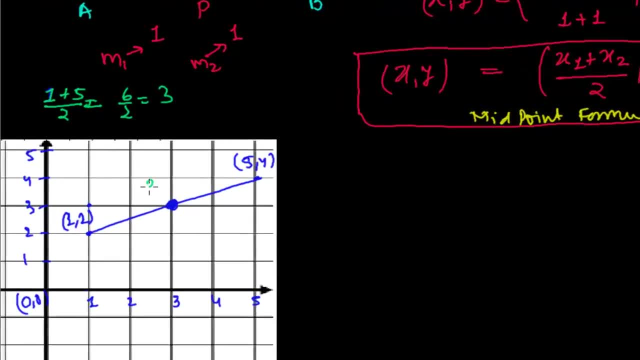 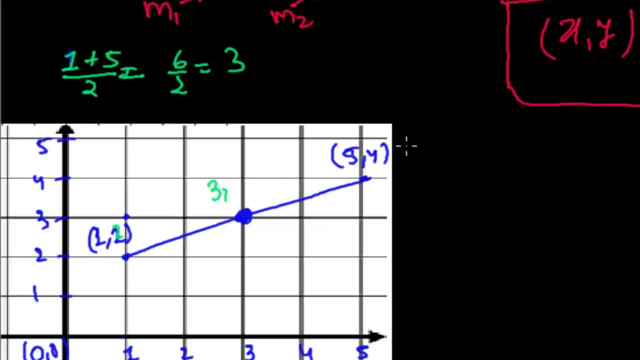 so x coordinate is now three again. average of this two and four, or i can say mean of this two and four again. let me take here two plus four divided by two, that is again four plus two. six upon two equals to three. so again i guard the value y, value three, right. so this is also three. 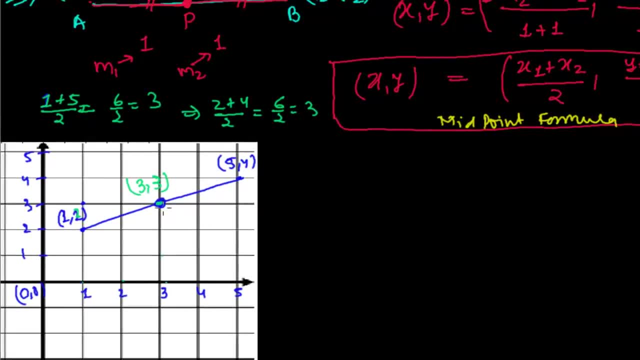 see here: one, two, three, one, two, three, so it's simply the average, right? it's a main point formula. it's just the average of two coordinates, right? just take the average of uh, the average of mean. you can say simply: uh, if you're learning the statistics, then it's simply the. 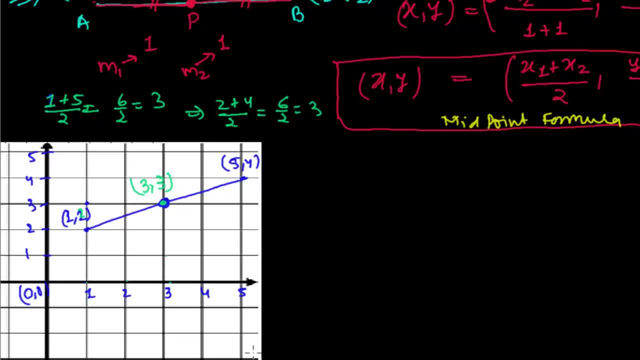 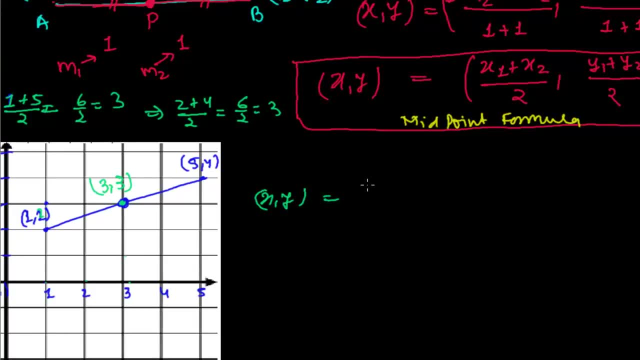 иб mean right. so if you just apply this formula again here, you will also get the same value right. see this i'm applying here. suppose this is x y, so x y. i will get right: x 1 plus x 2 upon 2, so x 1. 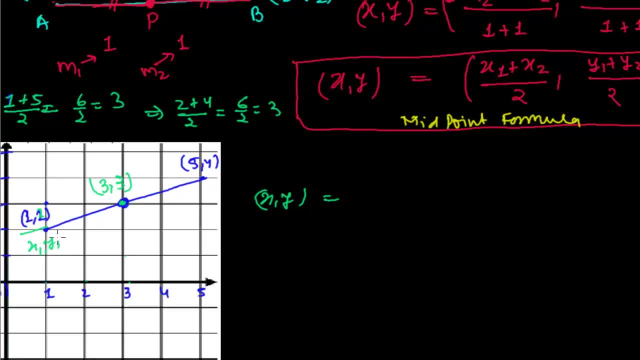 here is: let me suppose this is x 1 y 1, x 1 y 1, right, and this is x 2 y 2, right. it is working as x 2 y 2, so x 1 plus x 2, that is again 1 plus 5 divided by 2, and y 1 plus y 2, that is 2 plus 4. 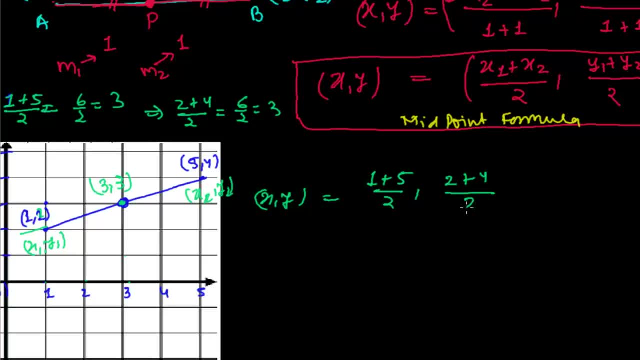 y 1 plus y 2, divided by 2, right is equals to right, 1 plus 5, that is 6 upon 2. 2 plus 4, that is 6 upon 2 right. so again, 3 coordinate 3 comma 3. so this is the midpoint of these two points. 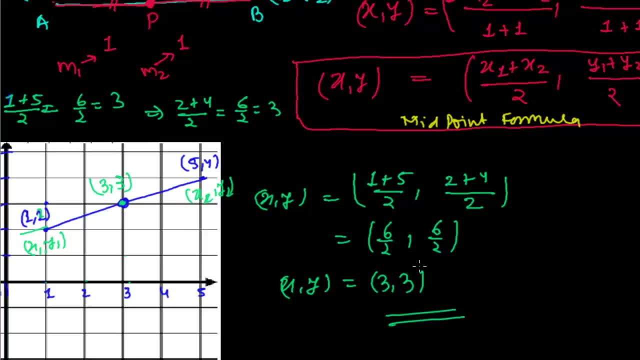 so, simply, this is called mid midpoint formula. exactly, it's nothing. just take the average of the coordinates right, take the average of x coordinate and take the average of y coordinate and the average that you got that is exactly the coordinate of the midpoint right in any line. 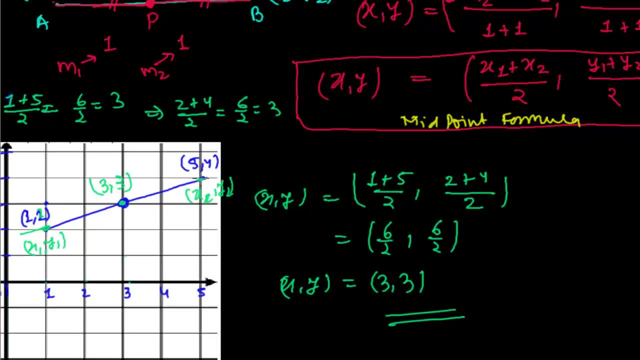 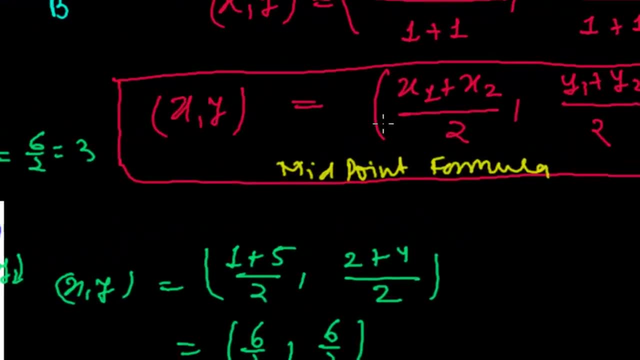 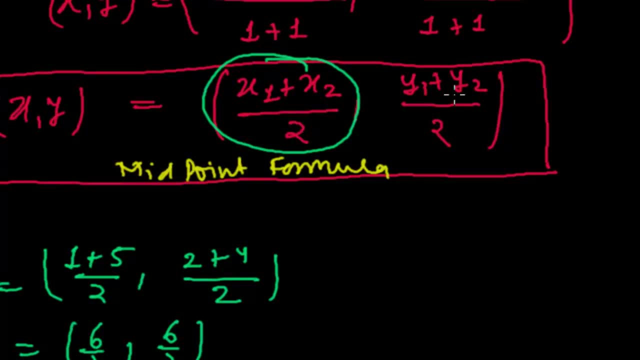 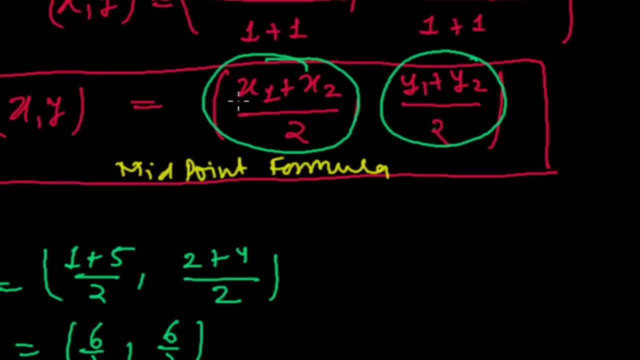 coordinates of midpoints. okay, so this is simply a midpoint formula. i think you now understand it and in next video we will be doing- uh, lots of problem related to this section formula and midpoint formula. okay, so keep watching on. we'll be meeting in next video. bye. 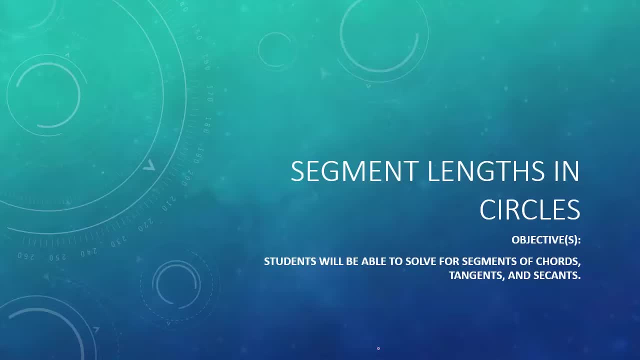 Hello, In today's lesson we're looking at Chapter 10, Section 5, Segment Lengths and Circles. Our objectives are to be able to solve for segments of chords, tangents and secants. We start with some theorem: Theorem 10.15.. 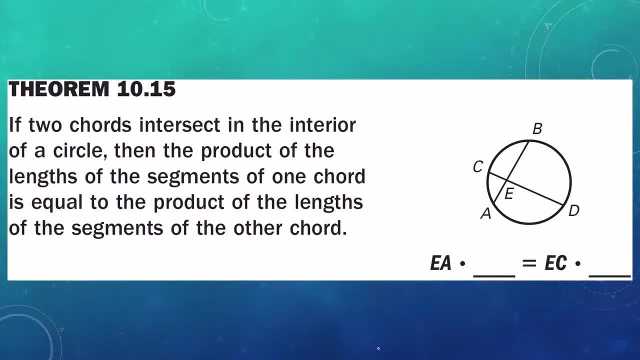 If two chords intersect in the interior of a circle, then the product of the lengths of the segments of one chord is equal to the product of the lengths of the segments of the other chord. That means that here we have chord B, A and C D. 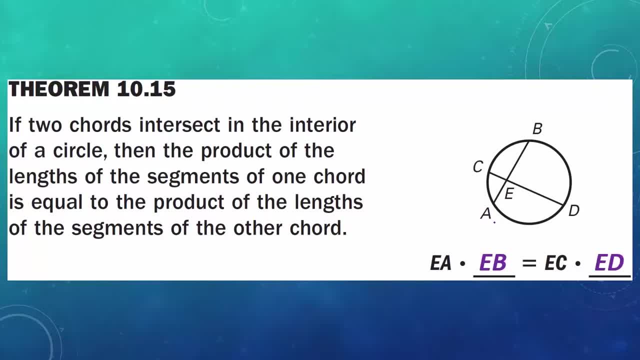 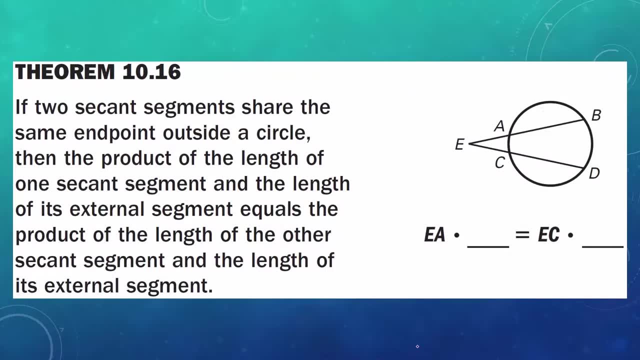 We can say that E A times E B is equal to E C times E D, Theorem 10.16.. If two secant segments share the same endpoint outside a circle, then the product of the length of one secant segment, 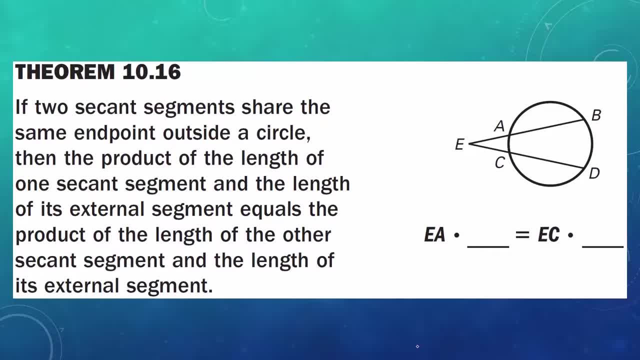 and the length of its external segment equals the product of the length of the other secant segment and the length of its external segment. So in this case, over here we've got two secants. We've got E B and E D. 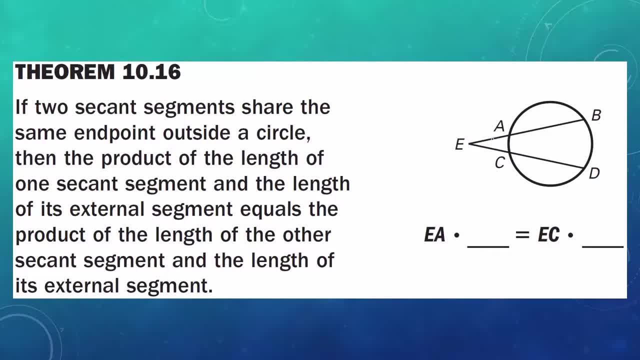 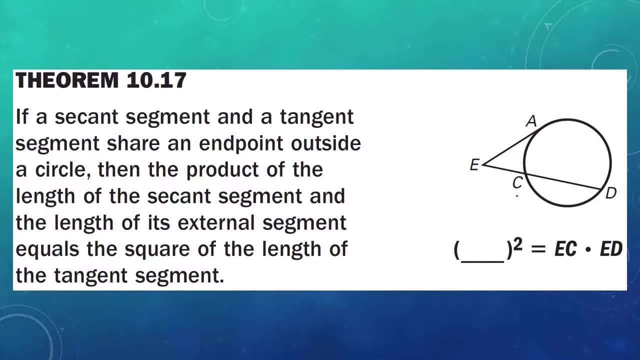 And their lengths are basically E A times the whole length. E B is equal to E C times the whole length of E D, Theorem 10.17.. If a secant segment and a tangent segment share an endpoint outside a circle, 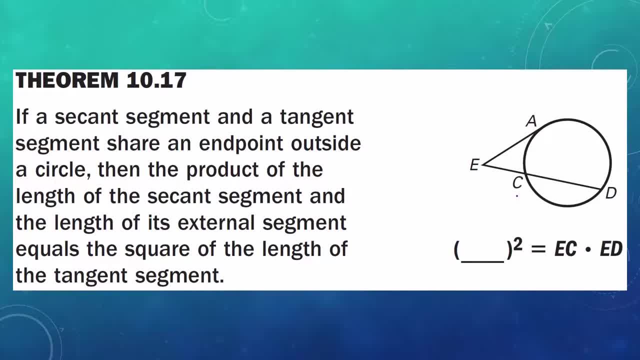 then the product of the length of the secant segment and the length of its external segment equals the square of the length of the tangent segment. So the tangent segment over here is E, A, So you're going to take the square of that. 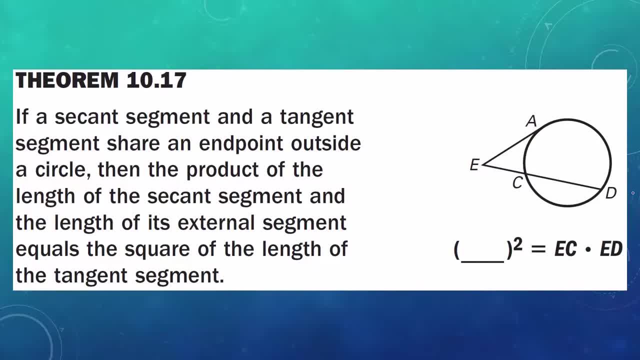 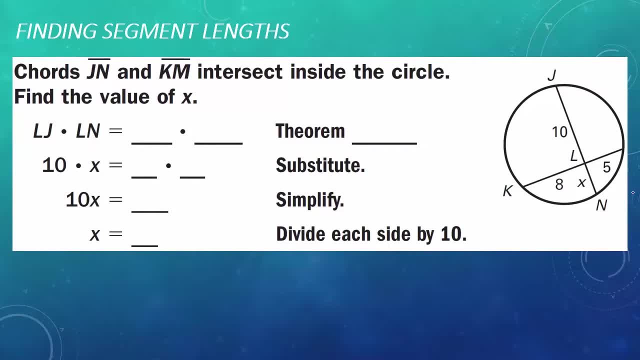 and that is equal to E C times the length E D. Example 1. Finding segment lengths. Chords: line segment J, N and line segment K M intersect inside the circle. Find the value of X. I can see J? N and K M.